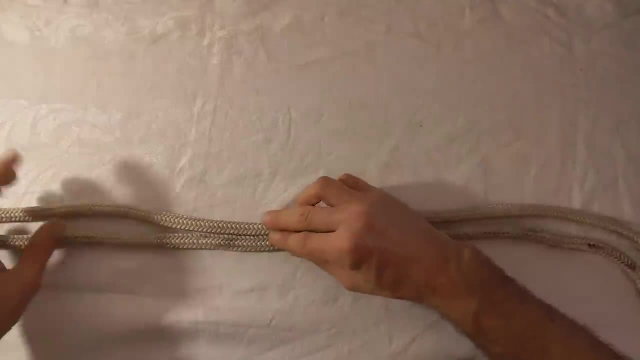 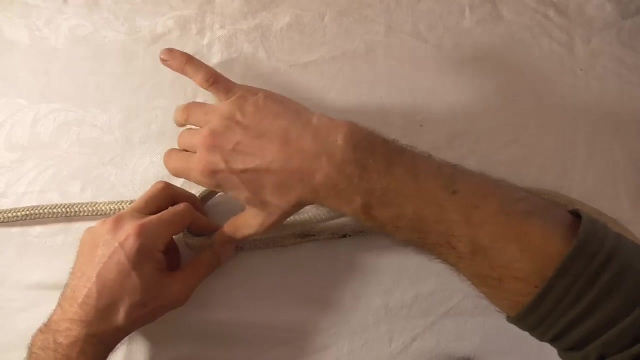 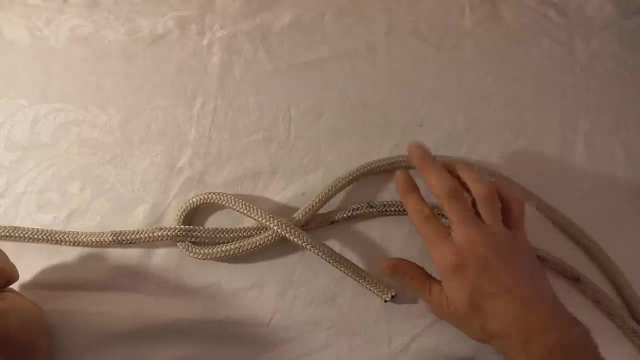 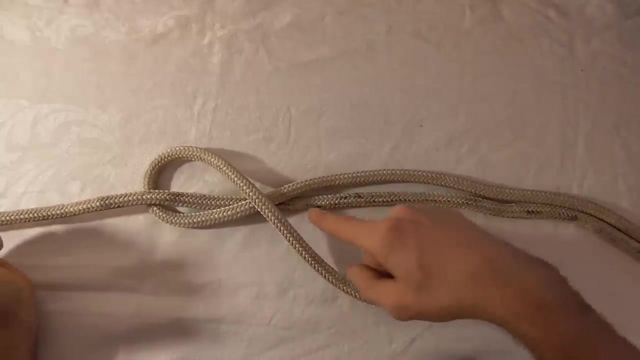 because we're going to need that rope to tie our knots and I want to take one end around the other like that, and it's going to make the shape of a Jesus fish. I'm just going to pull a little bit extra through Now. I want to take this: 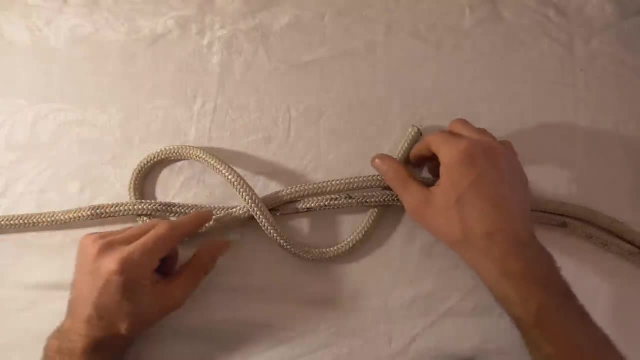 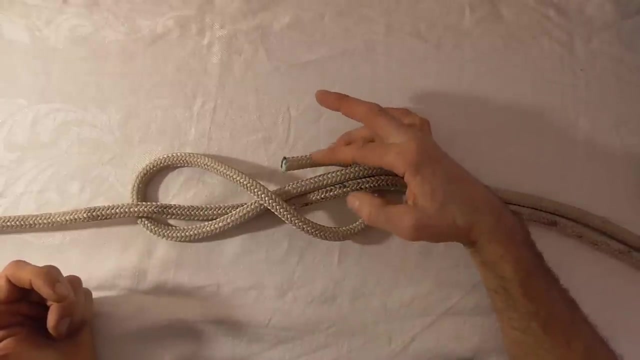 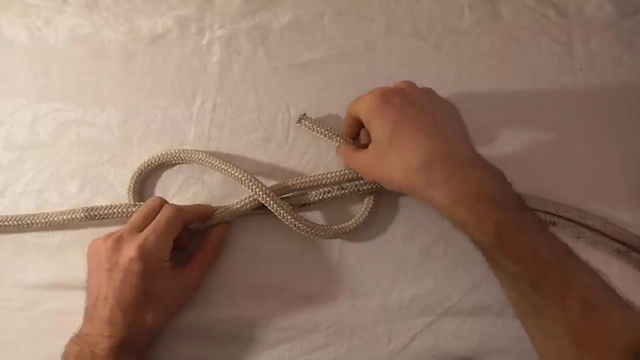 under both those parts there, so it's going to form the shape of an eight. I'm going to take this working end around the other end and I'm going to pull it up through both of these parts, and if you see this X here, I'm going to take it. 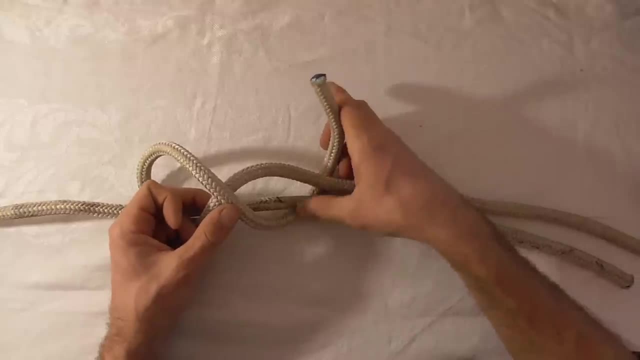 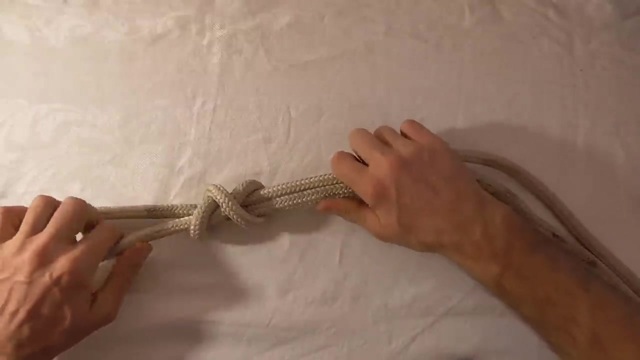 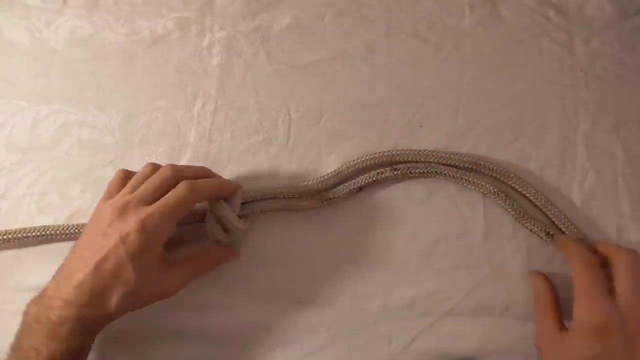 under that X, So around both these parts up through under that X and I can pull that tight and that forms a double overhand knot around the other rope. Now I want to do the exact same thing on the other side. I want to come around and 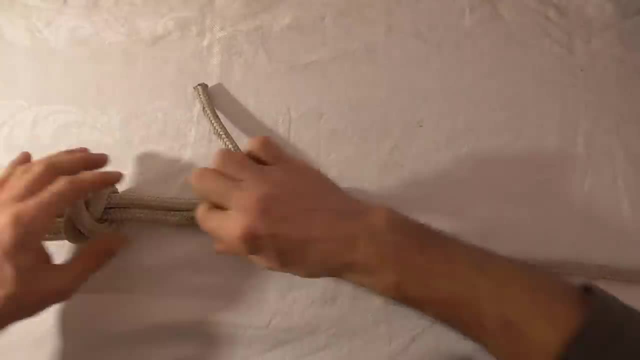 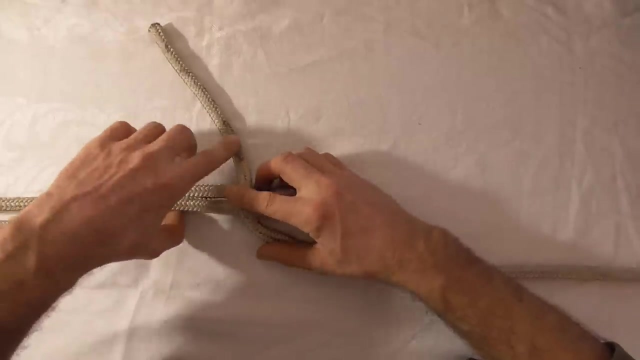 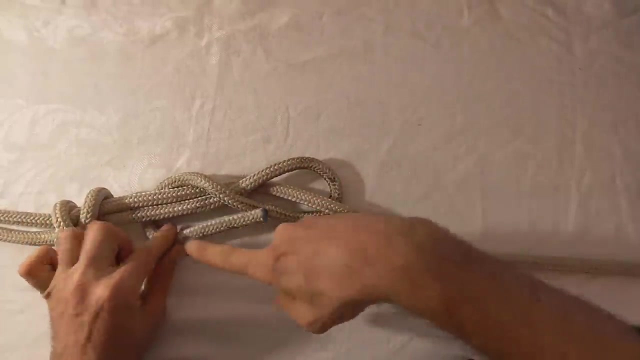 and make a shape like a Jesus fish. I'm going to give it a little bit of extra tail And I want to come around both these parts here so I can form my 8 shape. There we have this shape of an 8.. 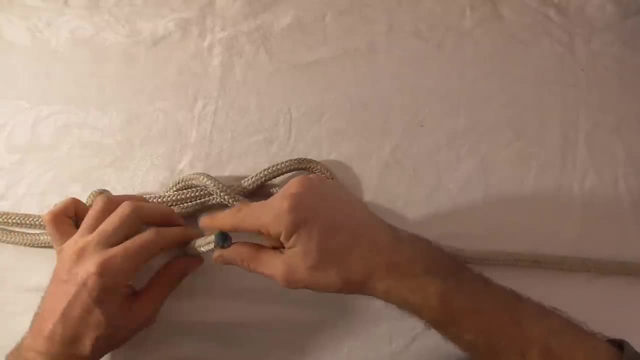 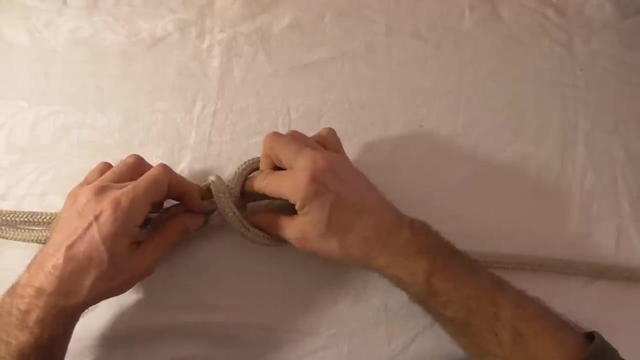 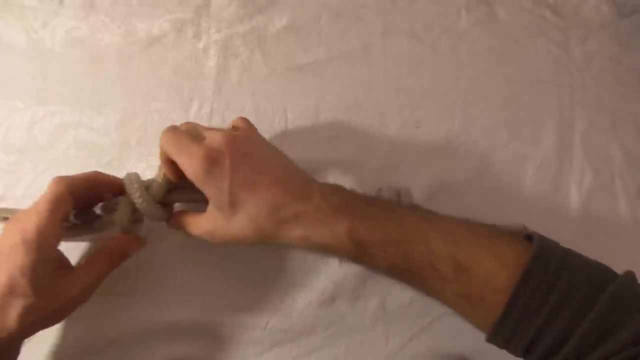 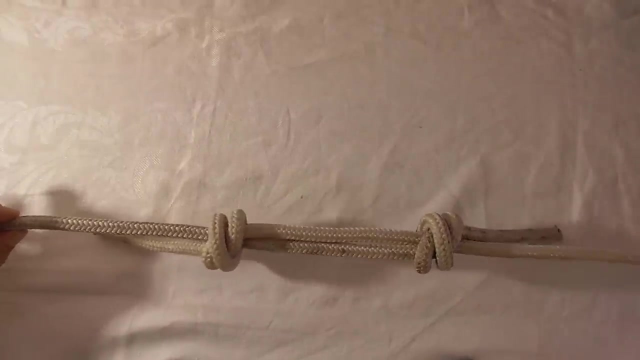 And I want to take this end around, both these parts, up through that X, Up through underneath the X, and pull it tight, Dress both knots. And now we can pull both these ends and these two knots will slide together. And if we pull really tightly these knots, 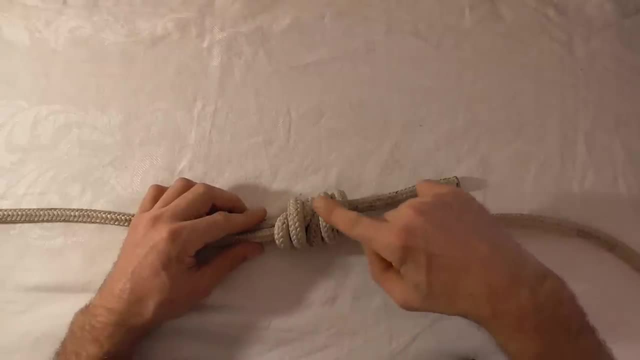 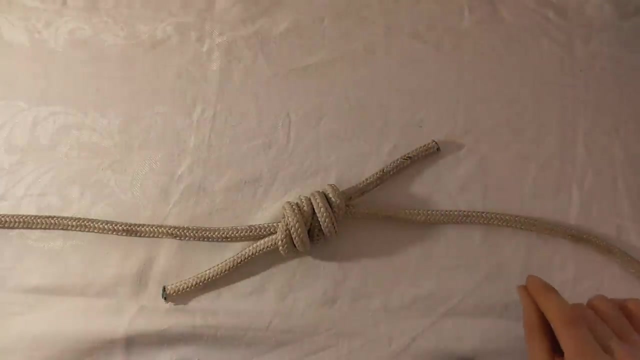 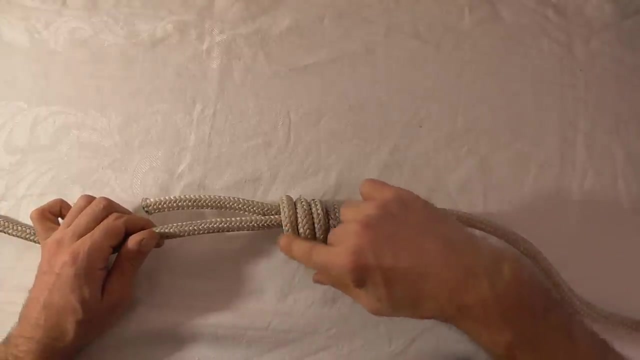 should set. Now, if we look at them, they should have two X's here Tails on opposite sides, And then if we flip it around, you'll see that these sides are parallel, And that's how you tie a double fisherman's knot.